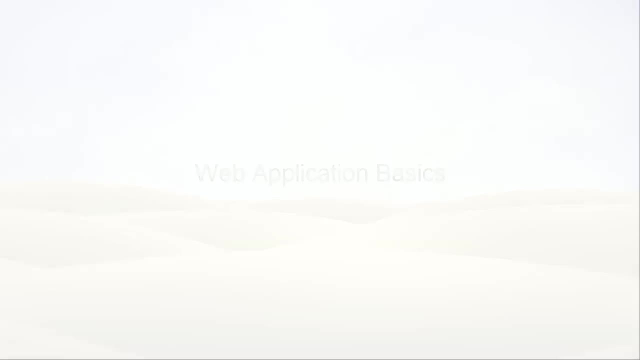 So in this video we are going to look at the basics of web applications, or how the web applications work. First of all, let's understand what's called a web application. A web application is a piece of software which can be accessed from a browser, And you know what's called a browser. A browser is an application that you use for browsing the internet, And the examples are your IE or Firefox. 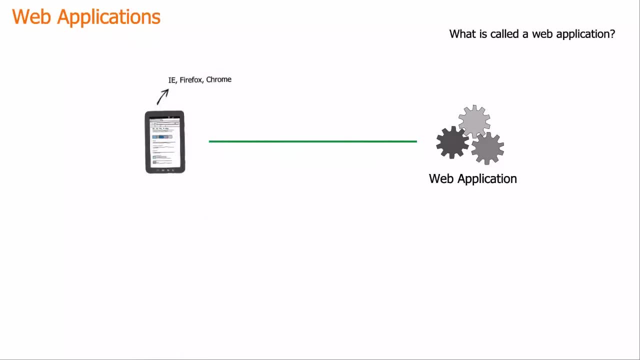 or Google Chrome or Safari. You all know about that. Technically speaking, we can call a web application a web server, Although there is a difference in the sense that a web server can host multiple applications. But for the time being let's call a web application a web server, And a web server is actually a network application running on some machine listening on a port. The browser is actually called a web client Or, more formally, we call that. 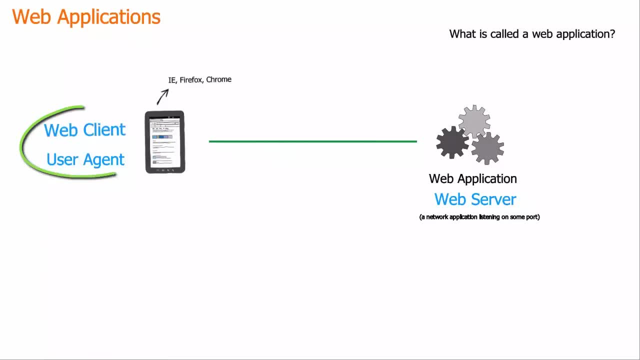 a user agent. And in fact web clients are not only browsers but any application which can speak to a web server, like your CURL or Telnet. Those are also web clients or user agents. So the web client or the user agent communicates with the web server to get its job done. And for this communication, and actually for any, 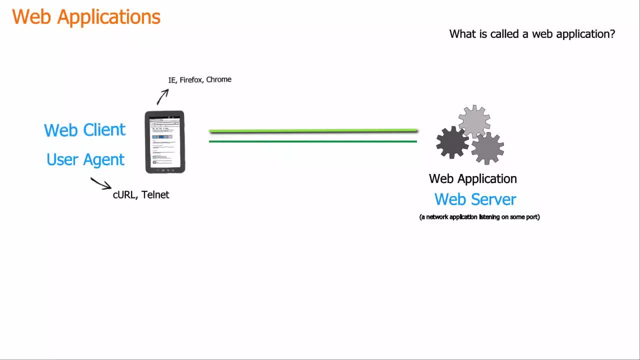 communication, both the parties needed to use the same set of rules or grammar, which we call protocol. in technical terms, you got what is called a protocol. it's simple, like when two parties are communicating. for example, when two people are communicating, they need to use the same language and the same set. 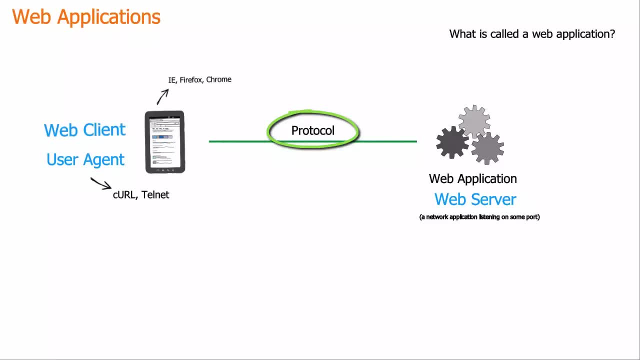 of grammar rules so that they can understand each other. similarly, in computer science, when two applications are communicating, they need to use the same set of rules, which we call protocol, and the browsers can speak some standard protocols like the HTTP protocol, the FTP protocol, the web socket protocol. there are many protocols which the browsers can speak. 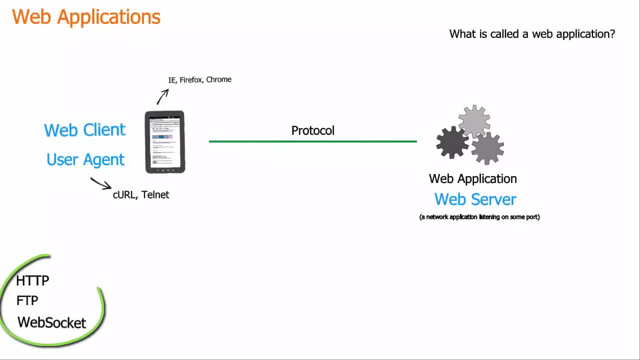 and they are standards and each of the protocols are suitable for different software such as Windows, Linux or Mac kind of tasks. for example, the ftp protocol is used for transferring files and among all these protocols the http protocol is the most used protocol in the web client and the web server club. 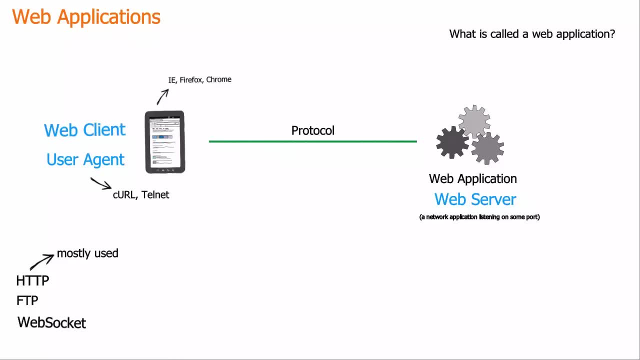 that means most of the times the web client and the web servers speak to one another using the http protocol and in fact, in this whole tutorial we are going to focus only on http protocol. so let's dig somewhat more into the http protocol. or to understand http protocol, we need to start. 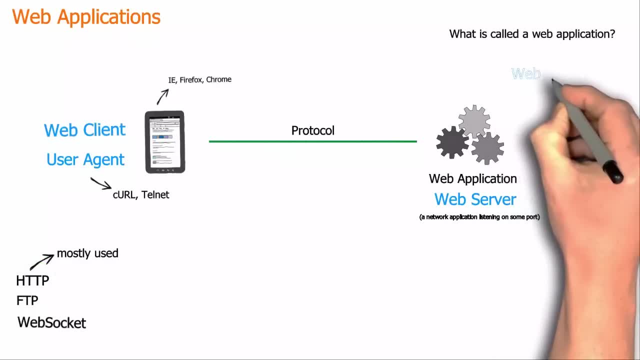 or let's start with what is called a web resource, or a resource, as commonly said. a resource is a document like an html document or a pdf document or a gestion document or an xml file or any kind of document which is hosted by a web server, or, in other words, a web client can access those documents through a web server. 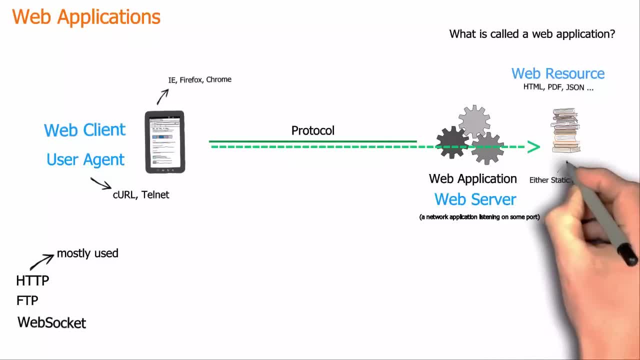 a resource could be either static or dynamic. a resource which does not change is called a static resource. that means it's like some static file sitting in the web servers hard disk or sitting somewhere which the web server has got access to and when a request for a resource 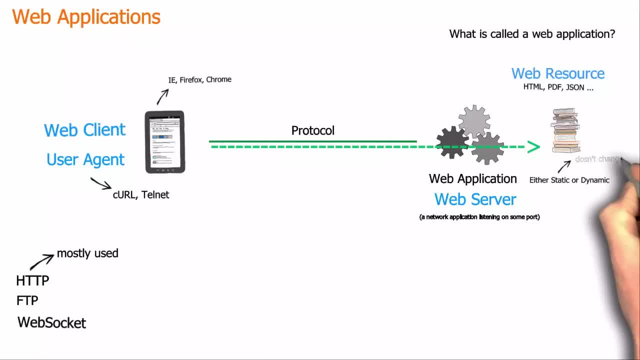 comes from a web client, the web server passes that resource to the web client straight. in contrast, a dynamic resource is generated on the fly, in the sense that when a request for a dynamic resource comes from a web client, the web server uh builds the resource on the fly. for example, 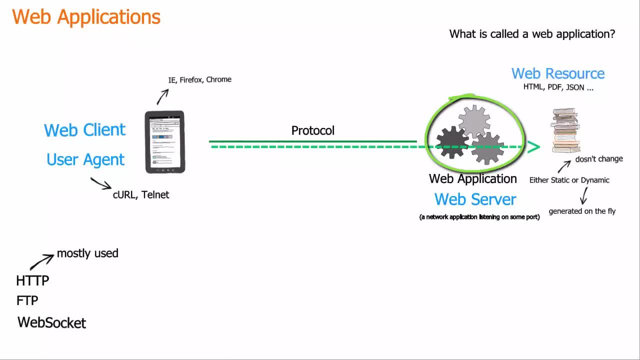 suppose a web server has a resource which embeds the current time either in a gestion or some xml document or an html page or whatever. so when a request for that particular resource comes from a web client, the web server gets the current time from the system and puts that into a gelsion document, bill suggestion document or an. 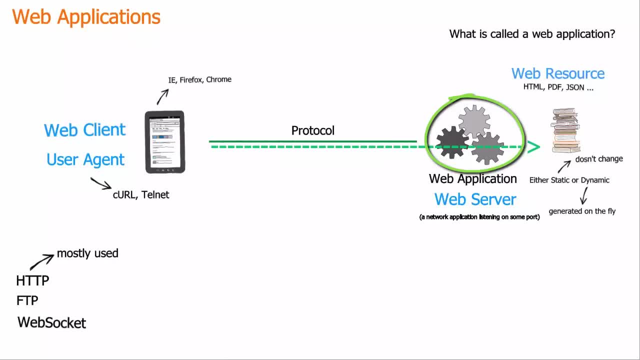 xml document or an html document embedding that particular time into it, and then it sends back that document to the web client. each resource on the web in the world is identified by a unique url, which is actually unique string. ah, it would be more clear when we look at an example. so this is an example of a url. 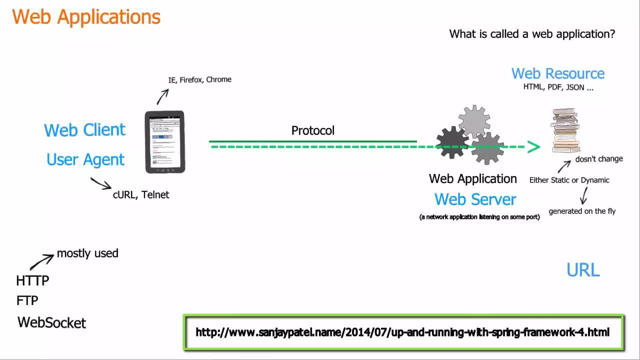 which points to a unique resource in the world, and this part of the url is the protocol and this part identify the web server in the world and this is the path of the resource in the web server. we will talk about url more in some later video. let's go back to http now. so http protocol is basically a request. 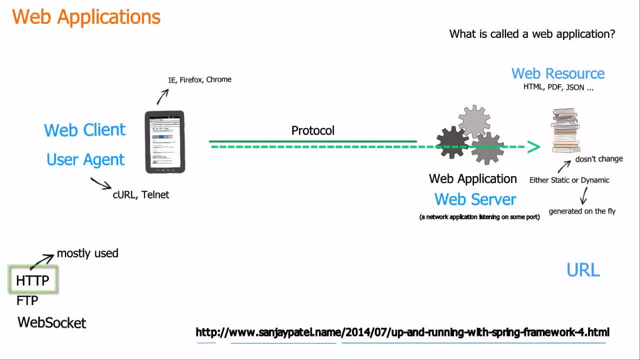 response protocol. that means whenever the web client needs to do some operation on a resource, like reading it or updating it or deleting it or creating a new resource or any kind of operation. the web plan first establishes a connection with the web server where the resource is hosted, and 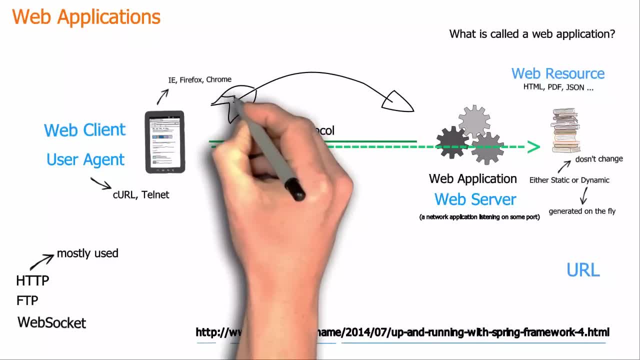 then the web client sends a request to it. the request contains the details of what the web client wants, like which operation it wants and all. while the web server receives a request, it responds with a response back to the web client. that means it sends a response back to the web client and the content of the response depends on. 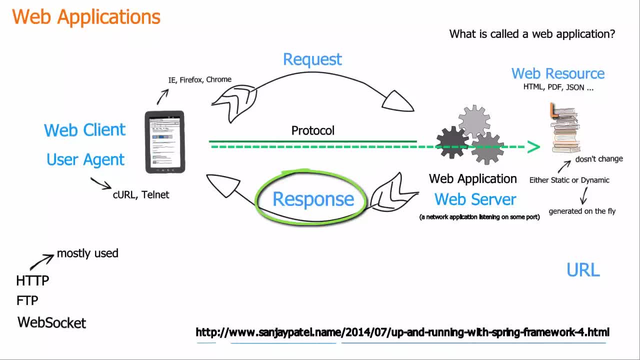 what was requested. For example, if the client asks to read a resource, the server can either put the resource in the response or inform the client that the resource is not available with me and you go to somewhere else for the resource, or something like that. 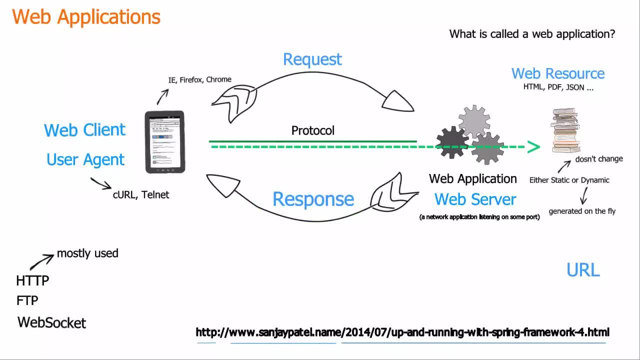 And then, after the response is given to the web client, the connection is closed and the web server does not remember anything about the past connections and who the clients were. That means next time, if the client sends another request to the server, the web server